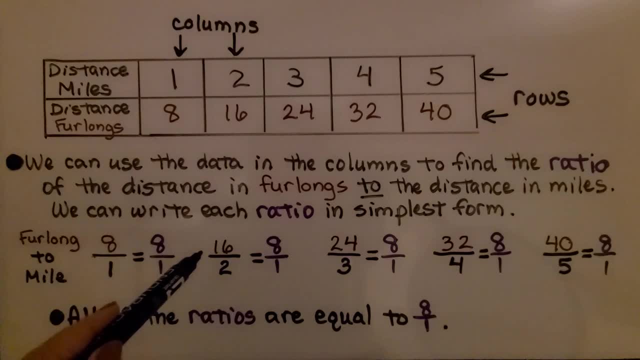 And if we have 16 furlongs to 2 miles, its simplest form is 8 to 1.. And 24 furlongs to 3 miles, in simplest form is 8 to 1.. They're all 8 to 1.. 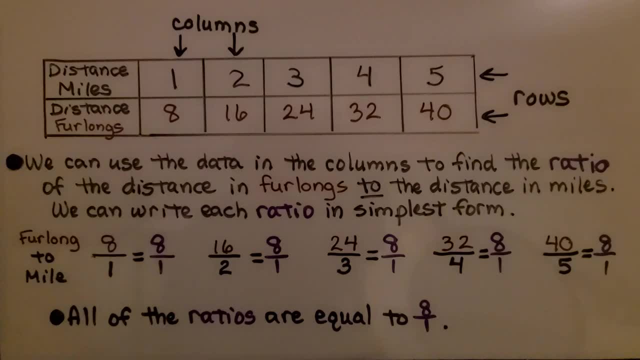 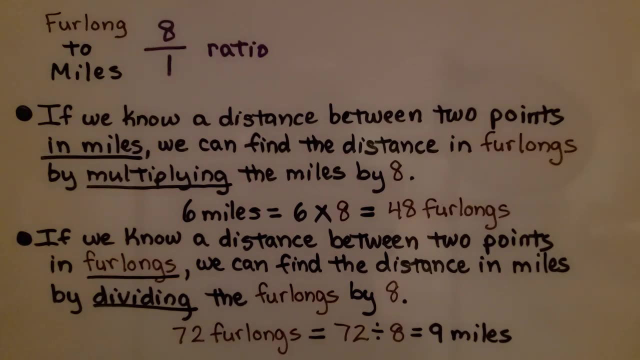 All of the ratios are equal to 8 to 1.. So for furlongs to miles, we have an 8 to 1 ratio. If we know a distance between two points in miles, we can find the distance in furlongs by multiplying the miles by 8.. 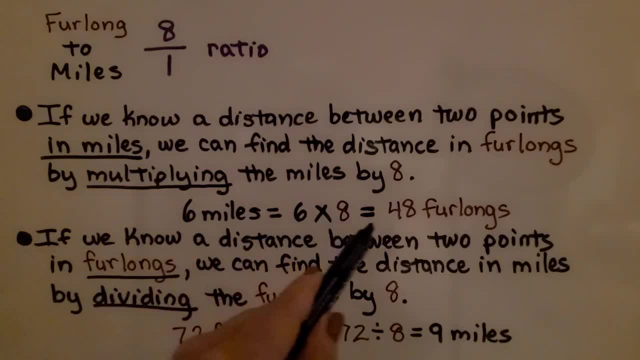 If we have 6 miles, we can just multiply 6 times 8.. And know that it's 48 furlongs. And if we know the distance between two points in furlongs, we can find the distance in miles by dividing the furlongs by 8.. 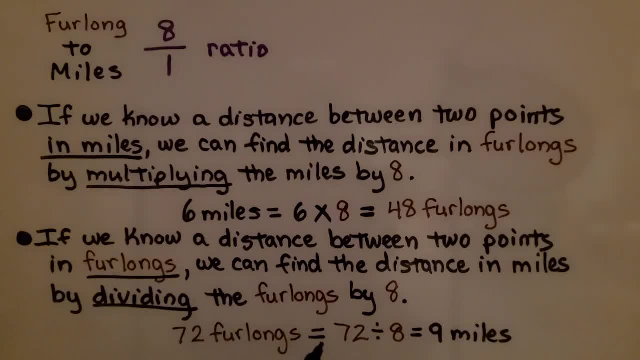 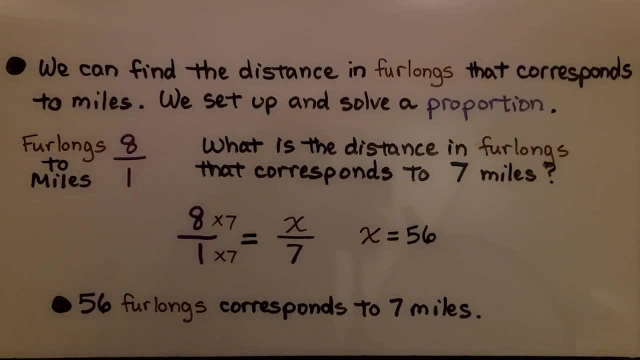 So if we have 72 furlongs, we know what it is in miles. by doing 72 divided by 8. That's 9 miles, We can find the distance in furlongs. that corresponds to miles. We set up and solve a proportion. 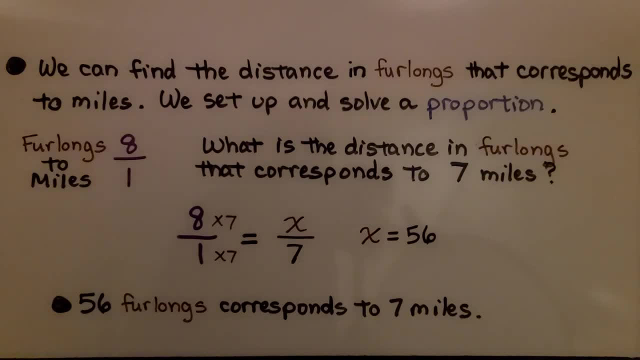 We have furlongs to miles. it's 8 to 1.. So what is the distance? We have a distance in furlongs that corresponds to 7 miles. We do 8 to 1 and x over 7.. We know 1 times 7 is 7, so we multiply the 8 by 7.. 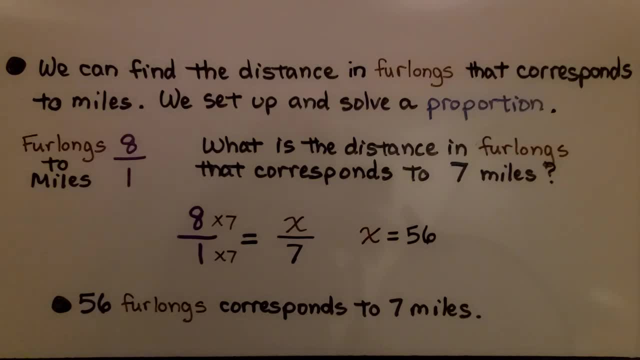 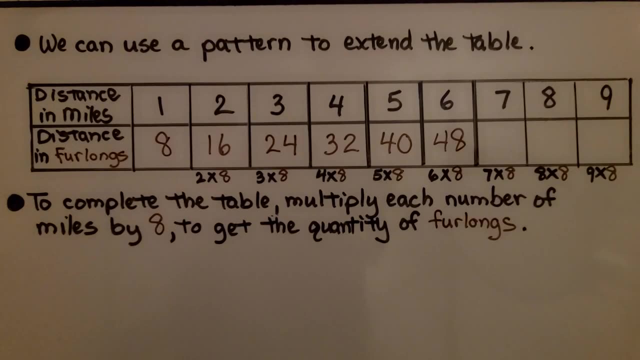 We get. x is equal to 56. 56 furlongs corresponds to 7 miles. We can use a pattern to extend the table. We have our distance in miles and our distance in furlongs. 1 mile is 8 furlongs. 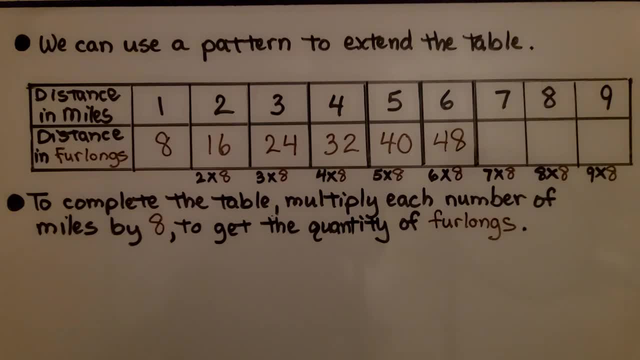 If we complete the table, we multiply each number of miles by 8 to get the quantity of furlongs, We have 7,, and 7 times 8 is 56.. We have 8,, 8 times 8 is 64. 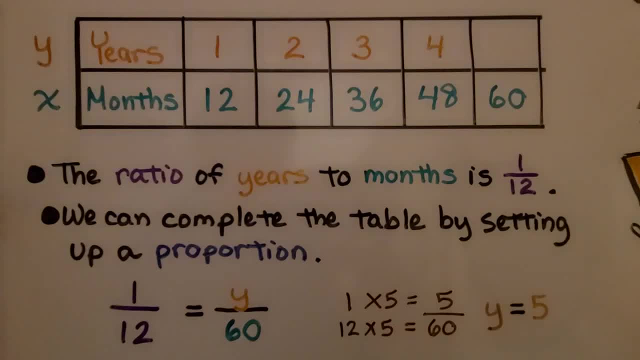 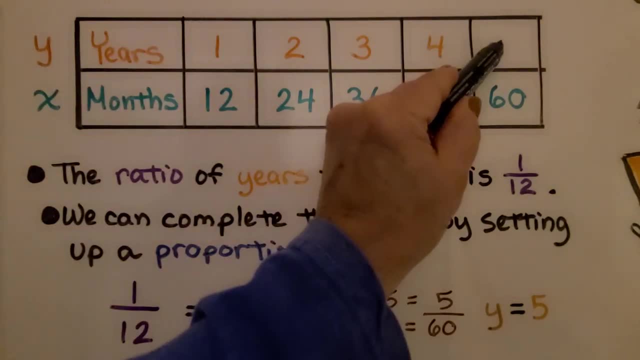 And 9 times 8 is 72.. Here we have a table and it's showing years to months. 1 year is 12 months, 2 years is 24 months and so on. But we're missing this one. The ratio of years to months is 1 to 12..